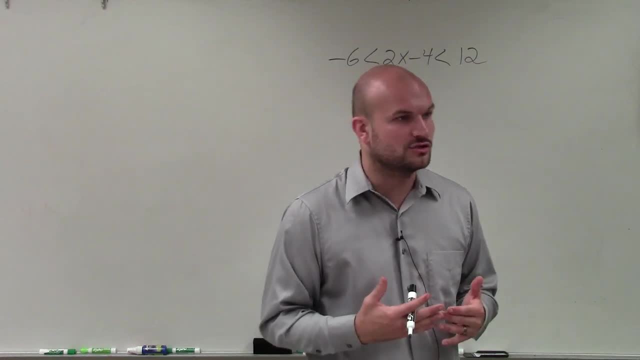 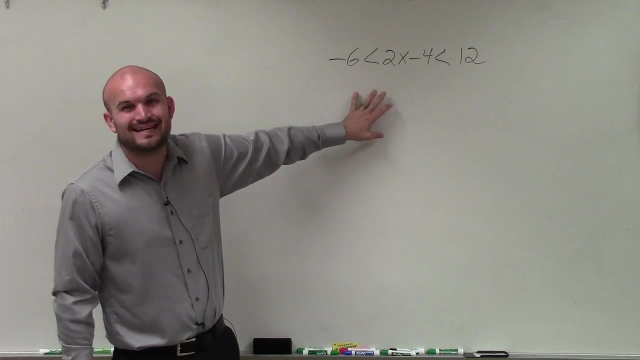 our solution usually involved more than one solution. So we went to our number line to represent the solution In compound inequalities. here's one way that we represented and compound inequality. So what I'm going to do is I'm going to show you guys kind of the longer 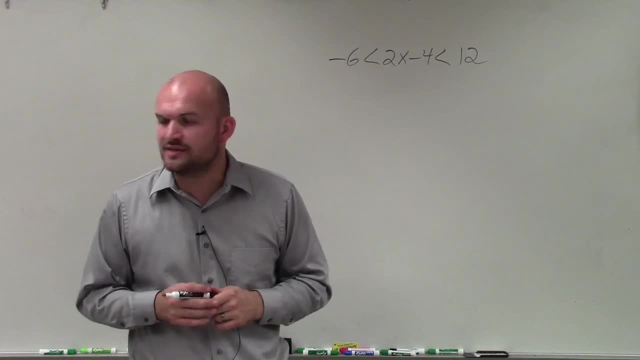 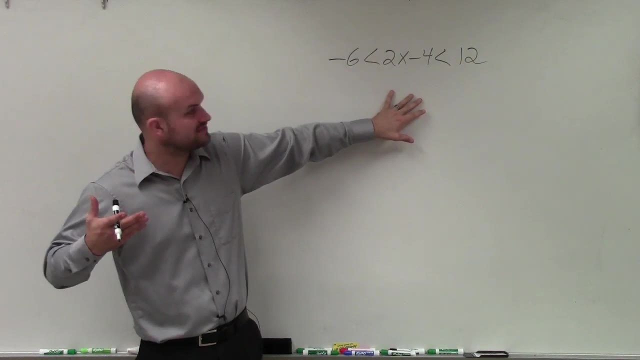 way to really understand what we're talking about, and then I'll show you kind of a different way to solve this as well. The first way that I prefer to have these solved, just for the understanding fact of solving them, is to break this up into an inequality with your. 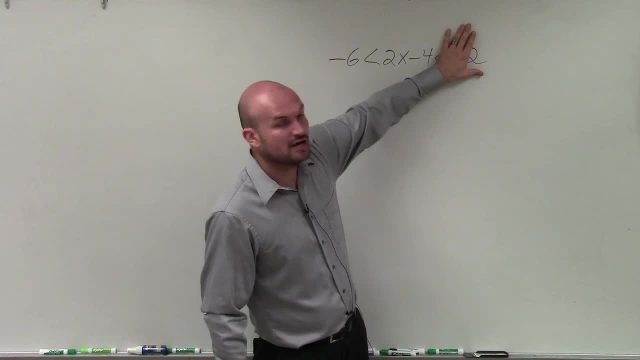 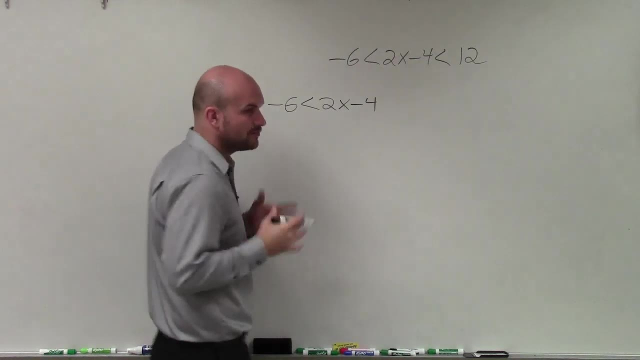 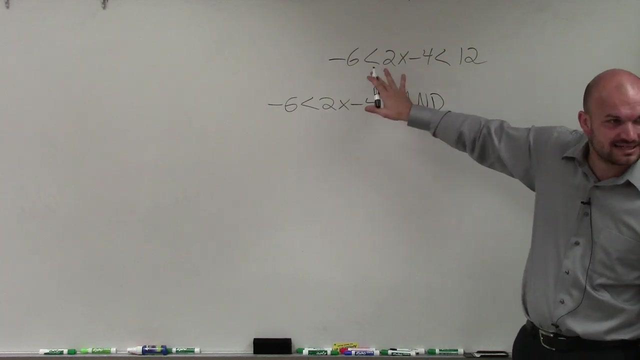 conjoining statement which is: and. So what we basically do is just cover up one end and we just write negative: 6 is less than 2x minus 4.. And the reason why I like breaking it up is because I like to use my conjoining statement. This is what we call an and compound. 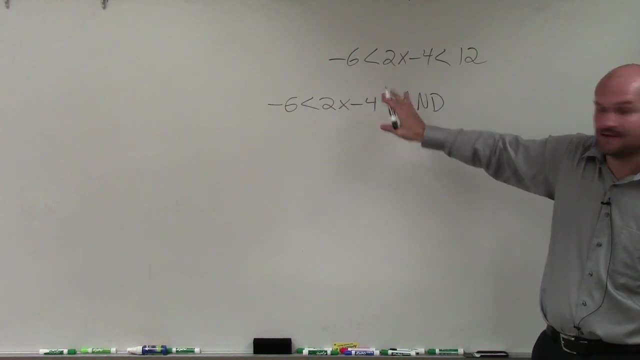 inequality And it's very important for Tansy, for you guys to see this, and So we're going to start with an and because when we talk about graphing and is going to become very important, So I covered this up. Now I cover this up And I say: 2x minus 4 is less than. 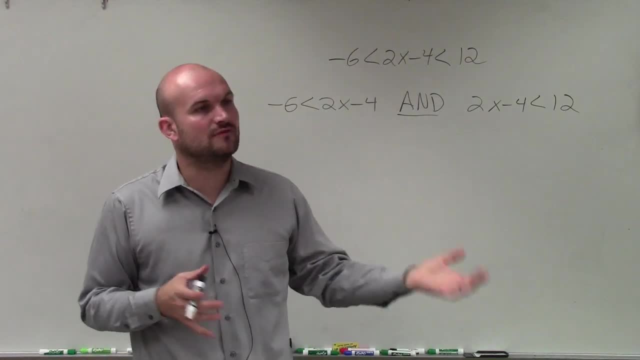 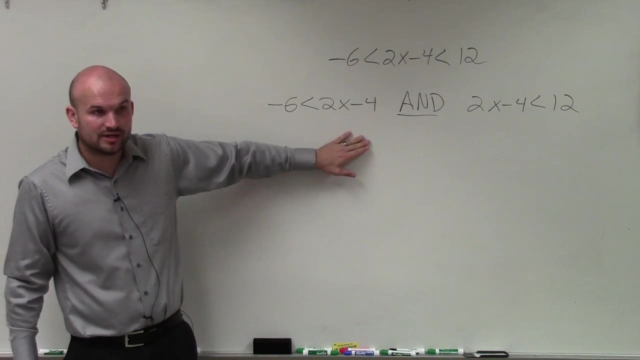 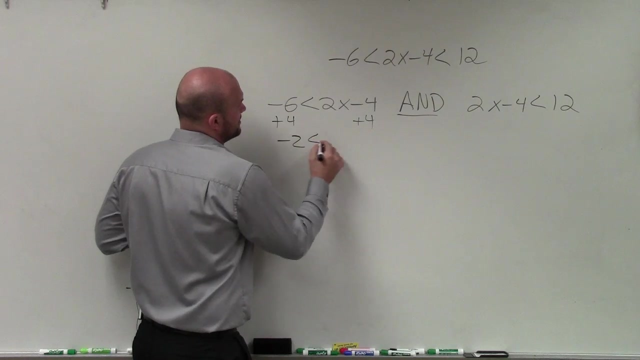 12.. So the middle part remains the same, It's just you cover up one side of the inequality on each end. Now I have two inequalities and I solved them just like we did last class period. I'll add 4 here. Add 4.. Negative 2 is less than 2x minus 4.. So I'm going to 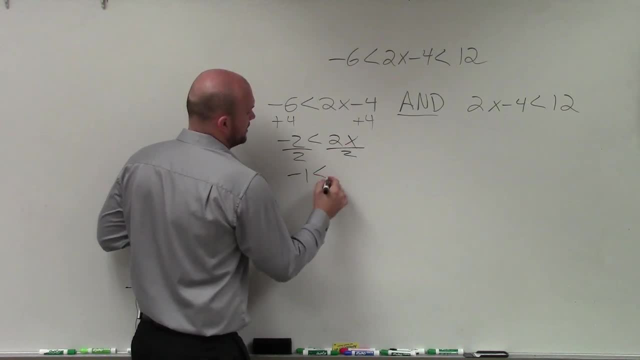 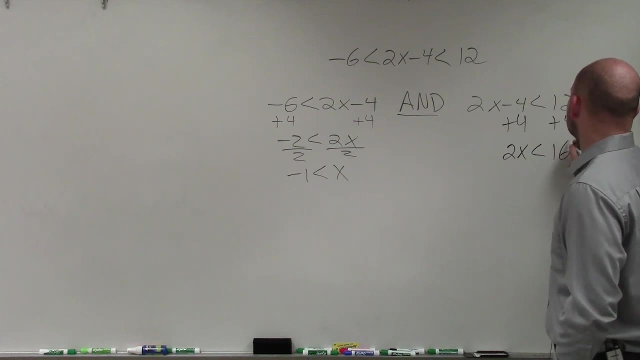 2x. divide by 2, divide by 2.. Negative 1 is less than x. Over here I add 4.. 2x is less than 16.. Divide by 2, divide by 2.. X is less than 8.. Now the issue though that comes. 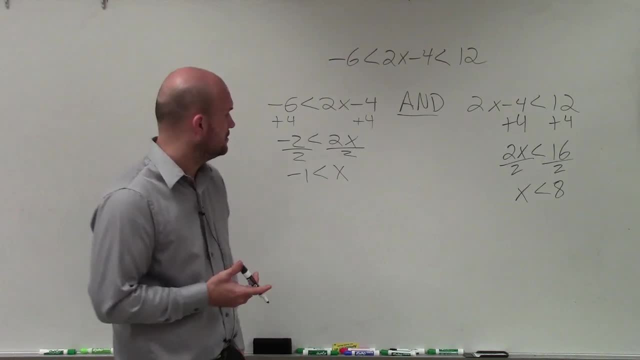 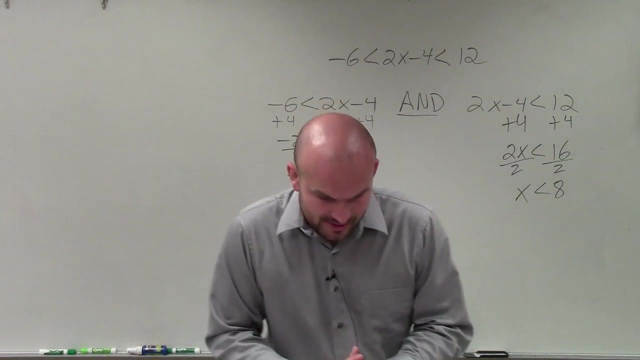 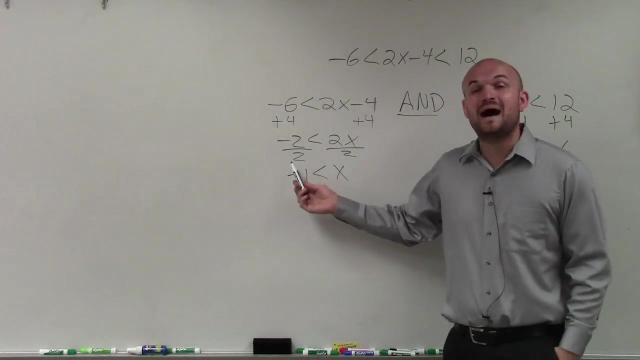 into solving it like this. Yes, So there's a couple issues with this. First of all is we need to remember we flip the sign when we multiply or divide by a negative number, And I'm going to try to do a problem that will be similar to that, But just notice, yeah. 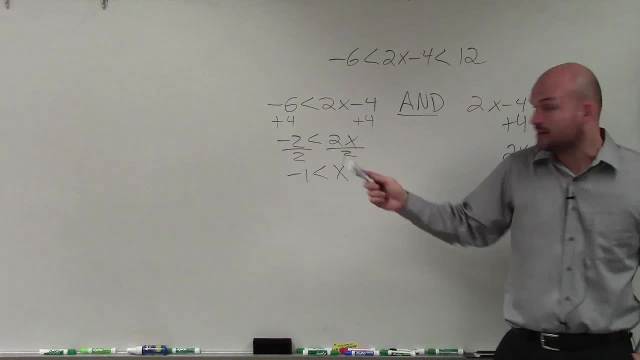 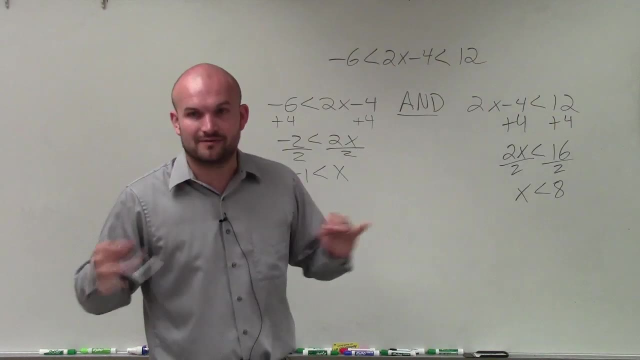 it's OK if I'm dividing into a negative number or multiplying into a negative number, But as long as my divisor or multiplier is positive, we don't have to flip the sign. It's only when the divisor or multiplier is negative that we flip the sign. The other problem with 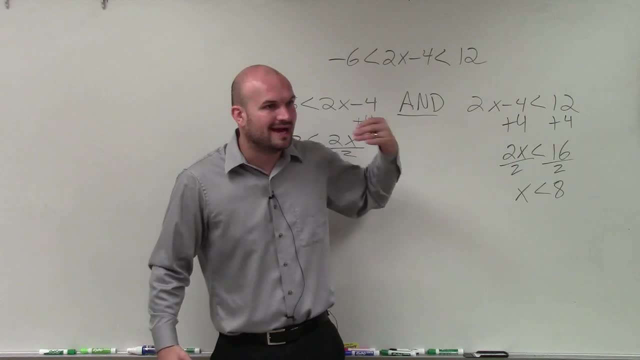 this is a lot of you guys might have gotten used to: oh, the graphing part, And a lot of times you have trouble with test points, Spending time doing test points, So you just say someone probably said oh, wherever the. 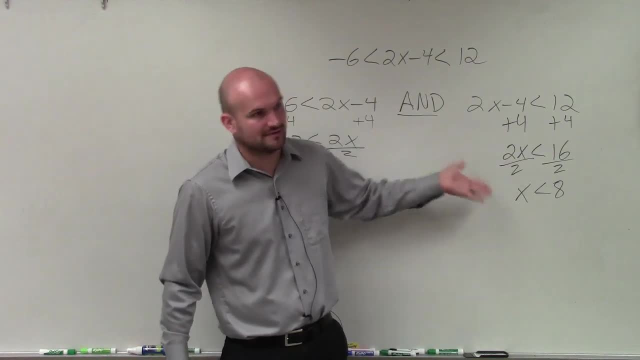 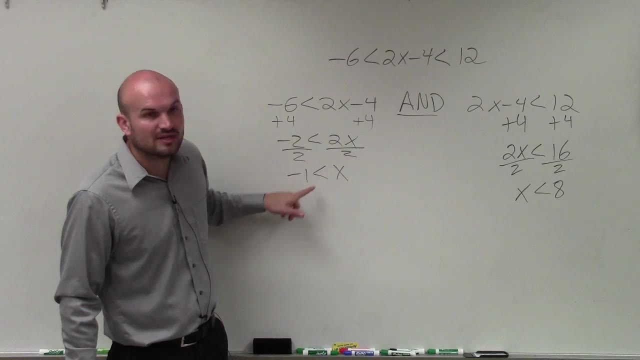 arrow's pointing, that's where you shade Right. It's like: oh, it's pointing to the left, So you shade to the left. And yes, for this one, that is true. For this one, that is false. The reason being is that it works when the variable is on the left side of the 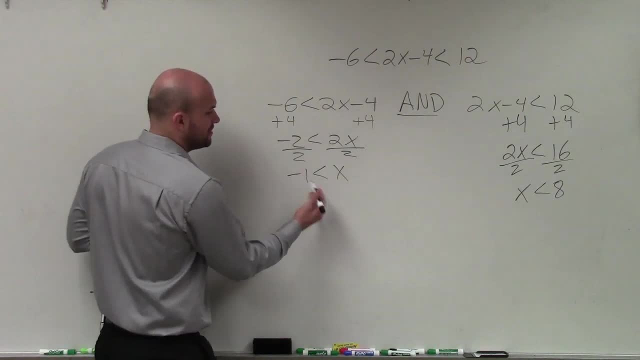 inequality statement. So one way you can do that is to flip this. inequality x is greater than negative 1.. OK, So these are the same thing. It's just now the variable's written on the left-hand side. So now we go ahead and graph. 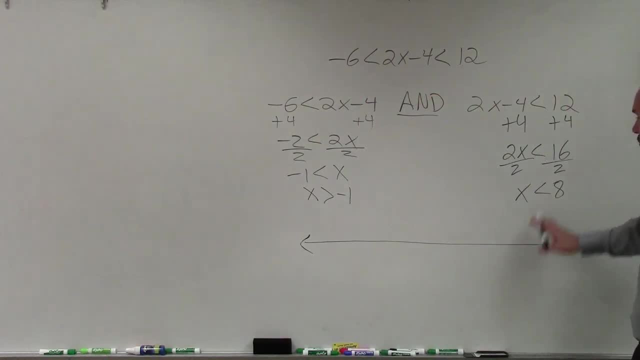 Now to graph this, I'm going to want to make sure I can include a number line that's going to include the number 8 as well as include the number negative 1.. So I'll do 10,, 9,, 8,. 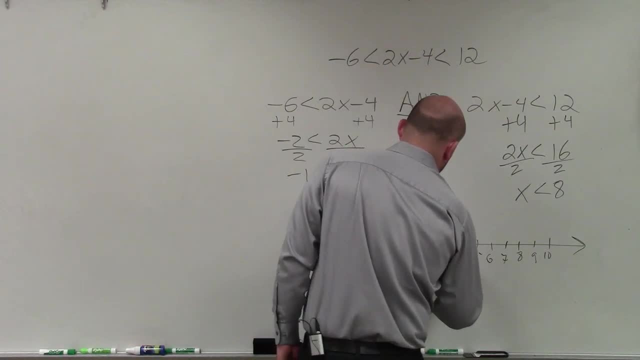 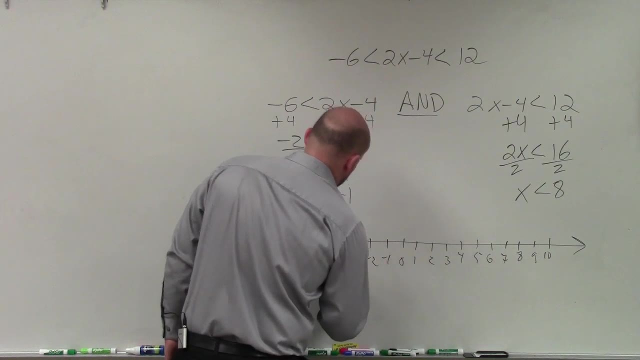 7, 6,, 5, 4, 3, 2, 1, 0, negative, 1, negative, 2, negative, 3, negative 4.. OK, I mean it's arbitrary guys, what your number line looks like. 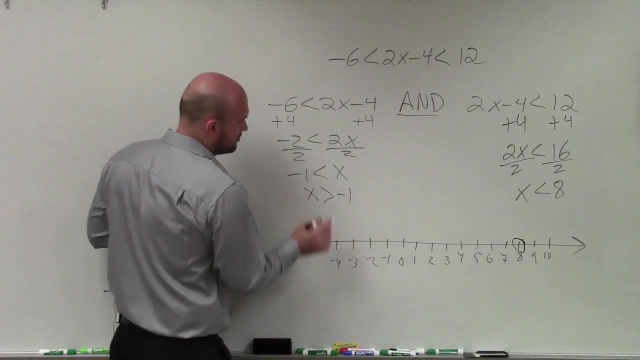 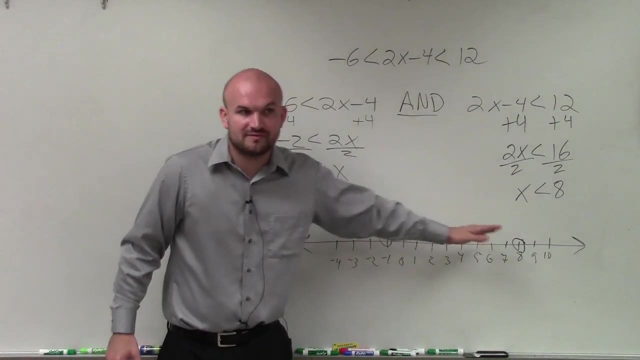 We just want to make sure we include points that are at 8 and include points that are at 9.. Negative: 1.. All right, Now let's look at the inequality symbols, because we could obviously use test points to determine if these are open or closed. 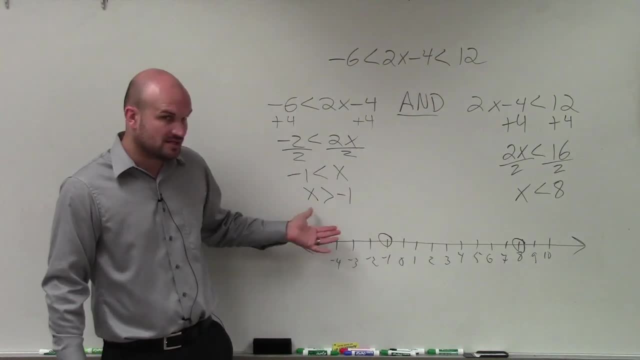 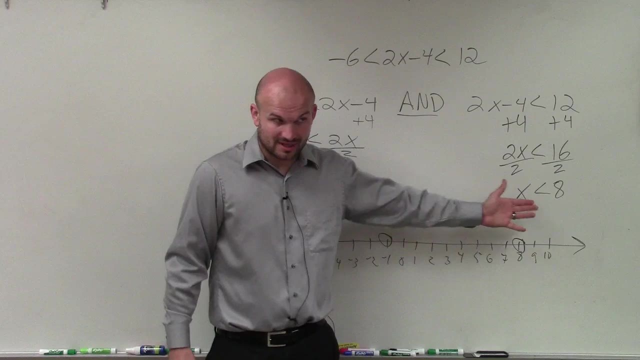 But I believe the easiest way to do that is just look at the inequality symbol And what we talked about two class periods ago. these are going to produce open or closed points. Open points: They are not a part of the solution. Let me show you again why. 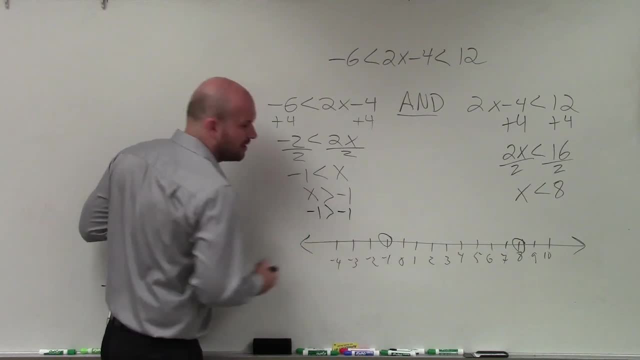 To make that true: negative 1.. Negative 1 is greater than negative 1.. Is negative 1 greater than negative 1?? Is negative 1 greater than negative 1?? No, It's equal to. So that's false. 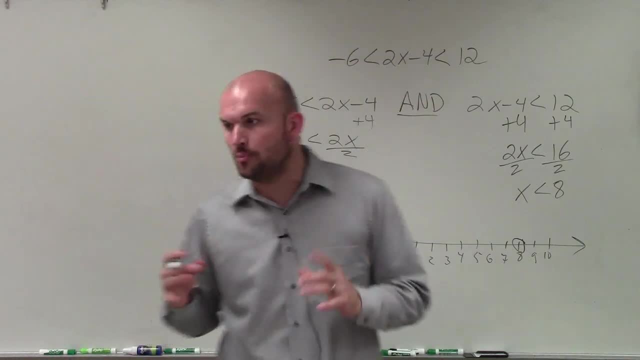 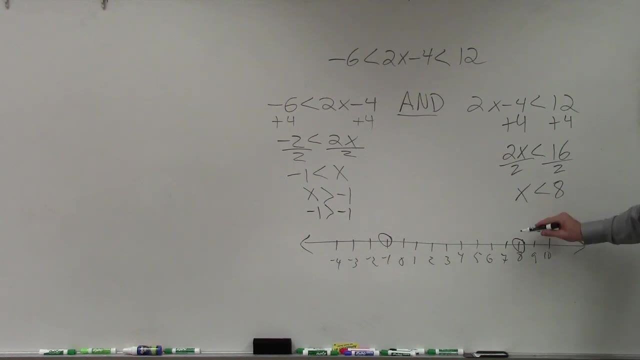 So that means negative 1 is not a part of the solution, So we leave it open. That's the same case over here. We leave it open. All right, Now I'll show you guys test points. next problem: For this problem it's just saying that x, this inequality, is true for values of x. that